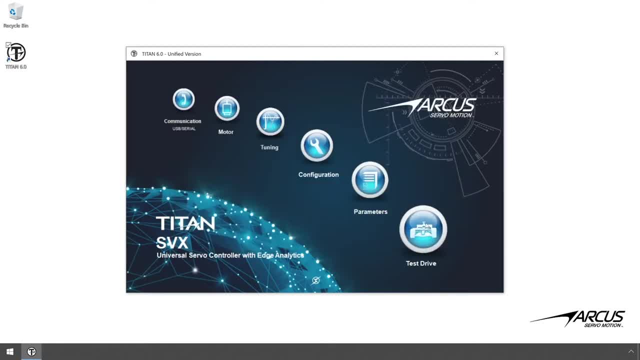 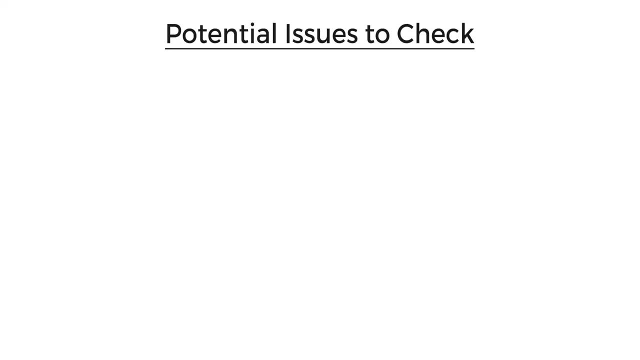 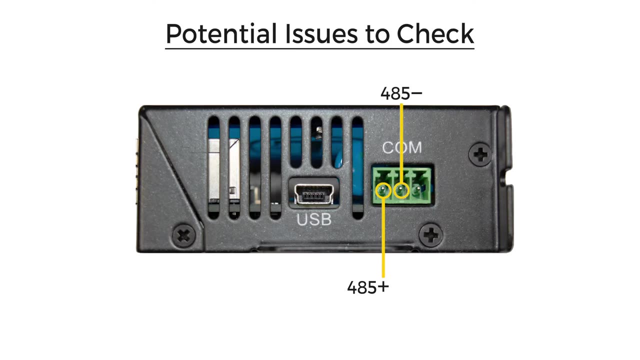 properly. You can try going to other screens and confirm the communication is working properly. Now, if the communication is not working, the following are the potential issues to check. First, check the 485 connections. Make sure that 485 plus, 485 minus and ground pins are connected correspondingly. Second, check the network ID and 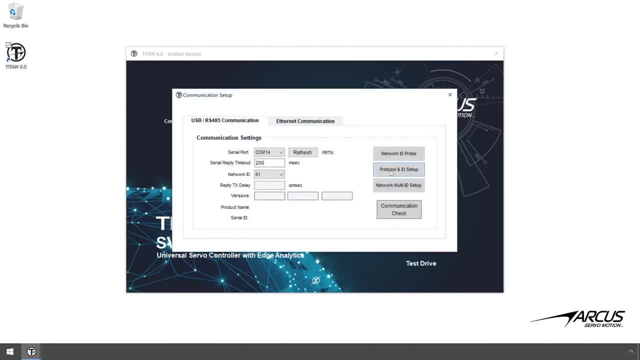 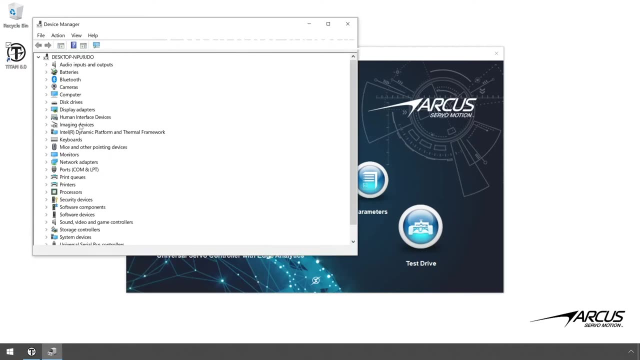 protocol. You can check the settings by opening the protocol and ID setup screen. When the Titan is shipped from the factory, the default network ID should be 1, with default protocol setting. Third, check again to confirm that the USB to 485 device driver is installed and working. 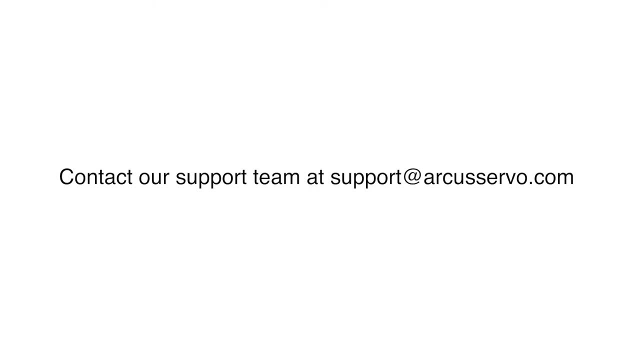 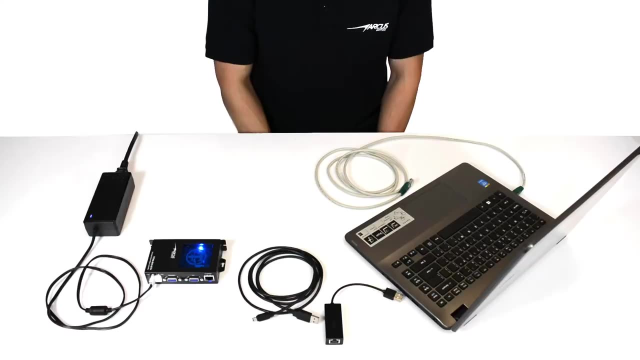 properly. If you're still having problems, contact our support team at Windows PC. Next, we'll communicate with the Titan using the Ethernet communication. Now, the Ethernet communication is going to be slightly different from communicating with USB or RS-485, so be sure to follow closely. First, confirm that the Windows PC has an Ethernet. 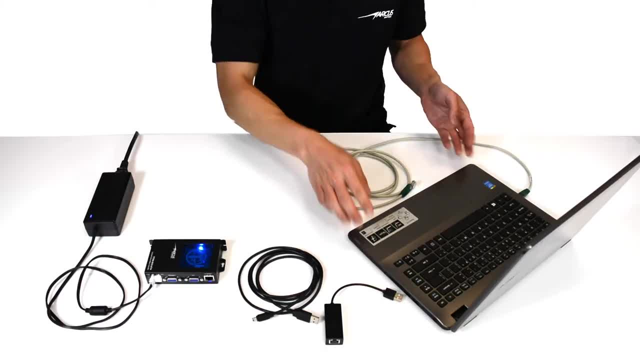 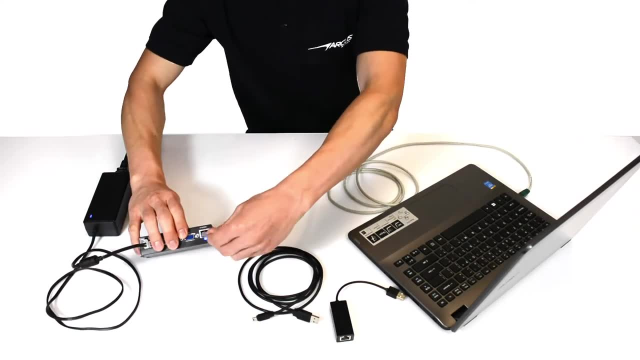 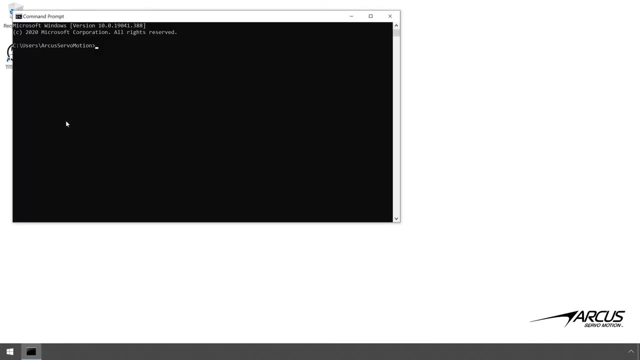 communication port, either built in, like this one over here, or using the USB to Ethernet converter. First thing to find out is the IP address of the Windows PC. Let's walk through on getting this information, Open the command prompt and type in the ipconfig command. 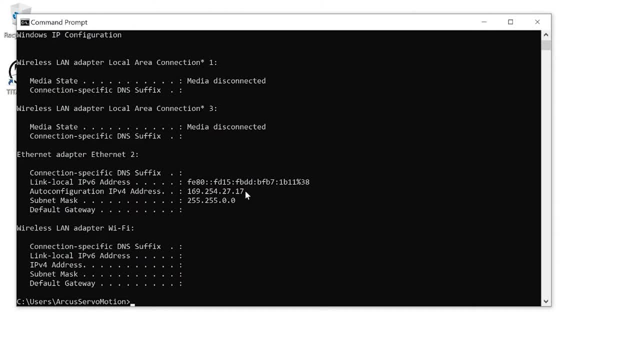 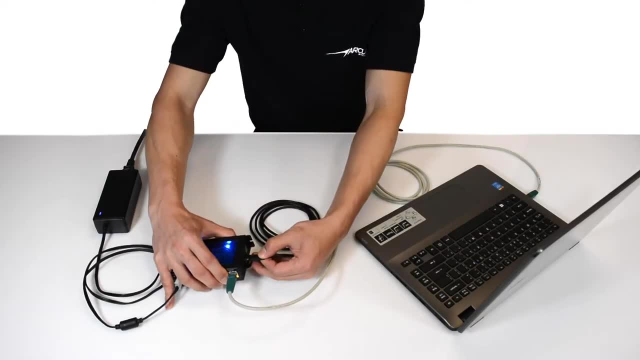 In the Ethernet section, you'll be able to determine the IP address of the PC. Next, let's configure the Titan's IP address so that it's in the same address network as the PC. In order to configure the Ethernet IP address of the Titan, you can use the USB or the RS-485. 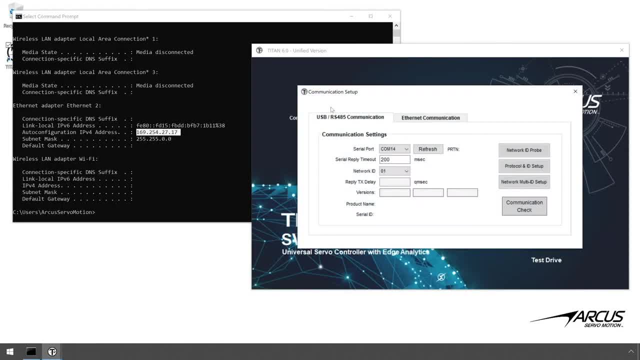 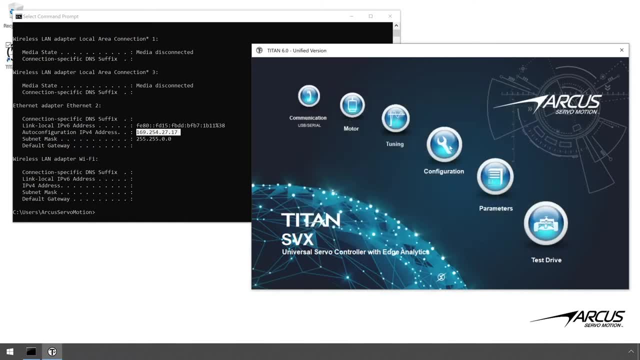 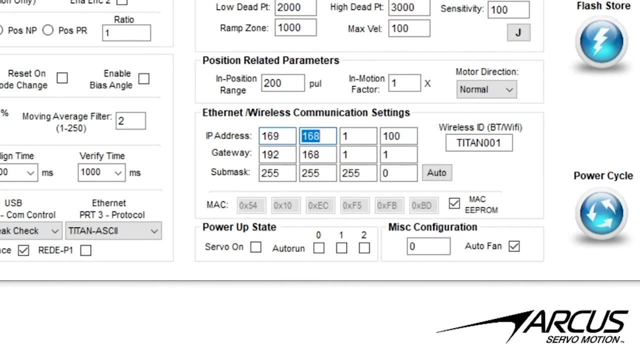 communication. In this example we'll use the USB communication and confirm that the USB communication is working. Next go to the configuration screen In the Ethernet section. enter the IP address of the Titan using the first three numbers of the IP address of the PC. For the last number, enter a. 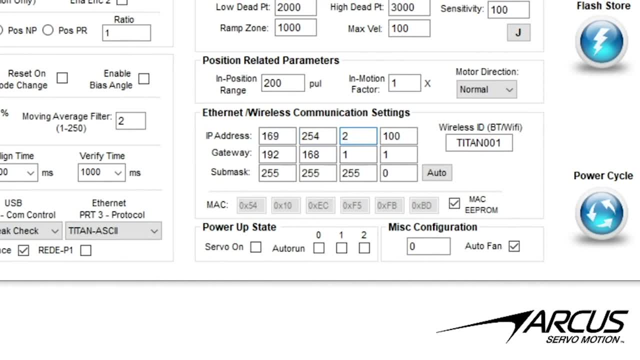 value that is different from the PC. For example, we'll use the value of 101.. Keep this IP address handy, since we'll need to use it later for the ping test, and in the communication section For the gateway, enter the same first three numbers and.